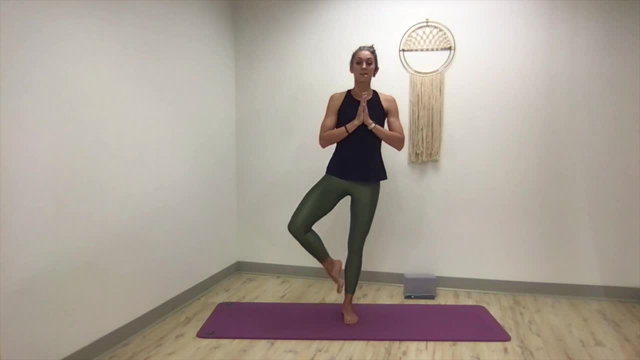 find the position that works best for you. So if that's toes tucked on the calf or upper thigh and then press down into the floor, Get rooted through your heel, through the ball of the toes, Press a foot into the leg and imagine you had a string attached to the top of your head that 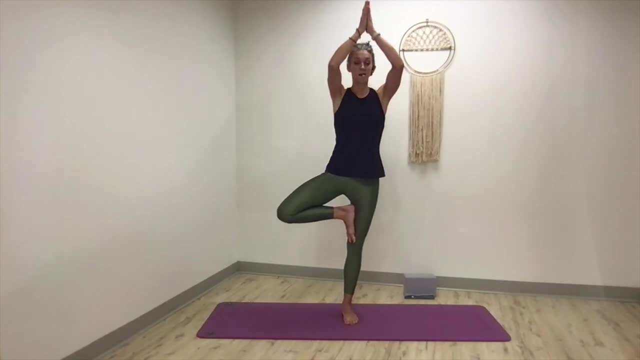 was pulling you toward the ceiling, reaching the arms up overhead. Lift your gaze, Find your breath. It's okay if you wobble here. It means you're challenging yourself. One more deep breath here. Inhale. bring the hands back together in front of the chest all the way down. 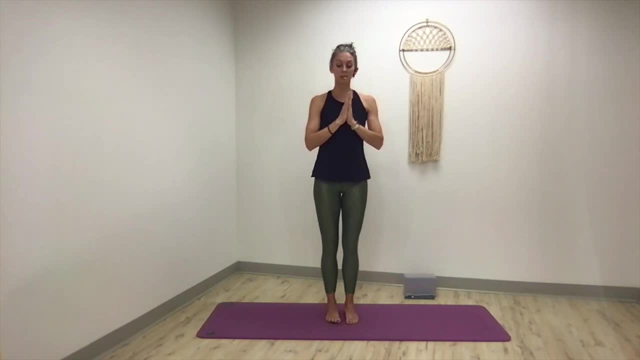 and replace your left foot back down to the floor. Release your arms coming into triangle pose. Step your feet wide, a little wider than where your wrists are bent. We're turning the right toes out, left toes in. to start, Take your left hand onto your hip. Reach your right arm forward. 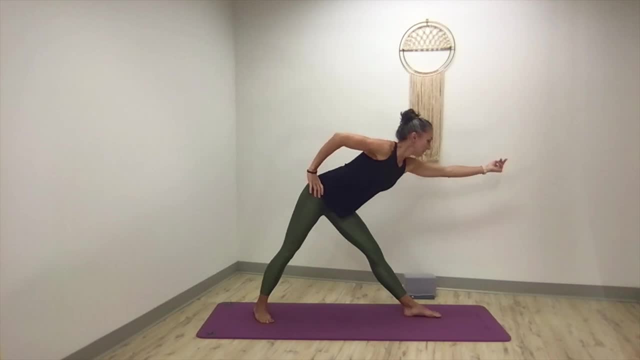 Draw back through that right hip as you're reaching. Imagine you're pulling yourself towards the opposite side of the room. Good, Now a block is really handy here. If you'd like to take a block here on the outside of your foot, you can take your hand to the block and take it to your shin. 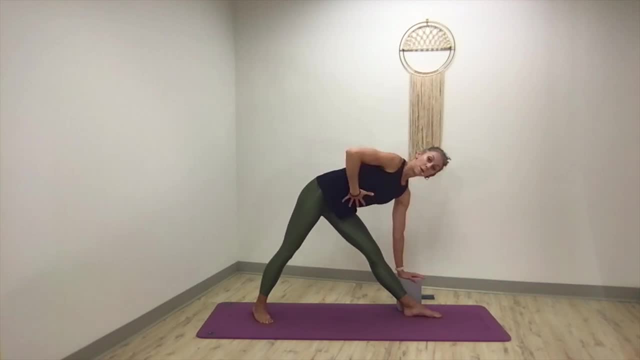 or to your ankle, whatever is accessible to you. Take a big breath in, Exhale, Engage your deep core and then maybe start to turn your chest towards the wall in front of you. Press down through your feet, Keep your spine nice and tight. 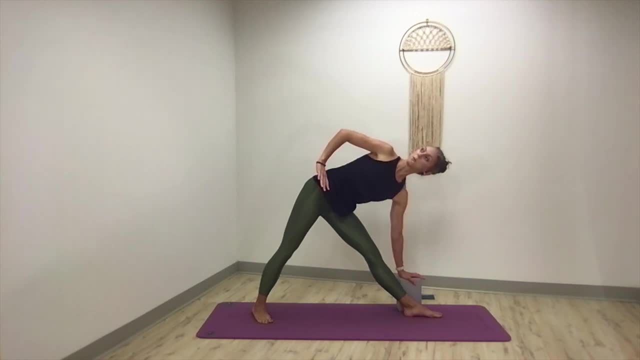 Nice and long. Use your core to help you rotate and open up through your shoulders, Press down through your bottom arm and then let that top arm float toward the ceiling. Your head can either be looking at your top hand, looking forward, or looking down. whichever is most comfortable. 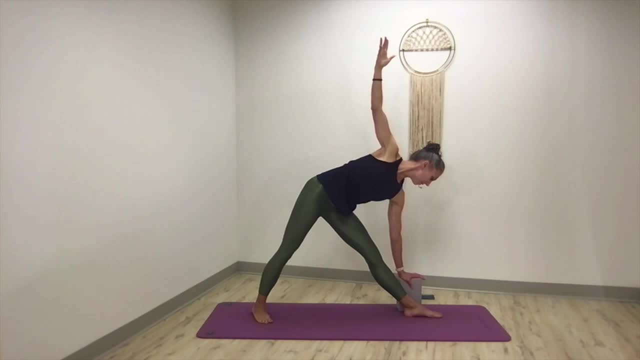 Deep, solid breaths here. Take your attention to your feet, Ground down through your heels and let that go. Let that reverberate up to your hips, through your tailbone and elongate through the crown of your head. One more breath here. Exhale Left hand to your hip. Grab your block if you have it. 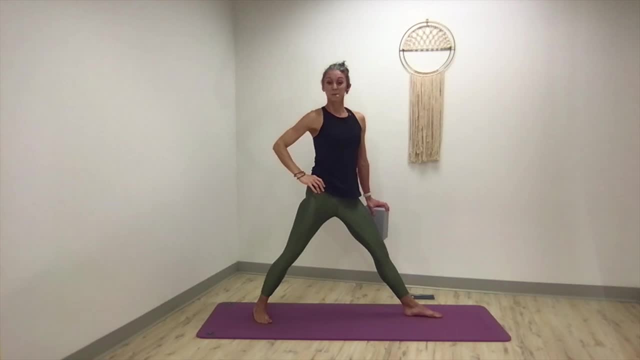 with you. You're going to press through your left leg. Come all the way up to stand and we'll switch sides, Turning your toes out, Left toes out, right toes in. Switch the hand with the block, Reach the arms out With that block. you're going to reach towards the left. Really, drop. 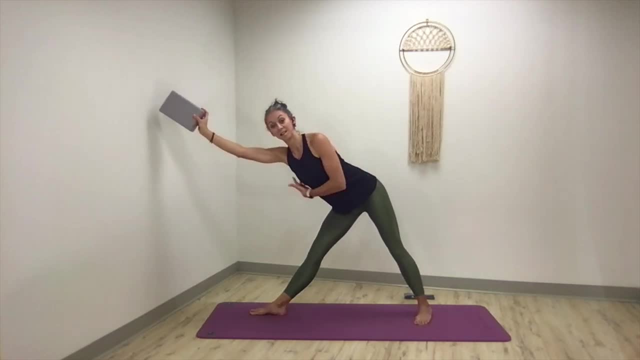 into the ground To that hip, find the spaciousness here and lengthen the side body And then drop that arm all the way either down to the block, to the floor or to your shin or to your ankle, wherever is accessible to you, Good. Elongate through your ribcage. 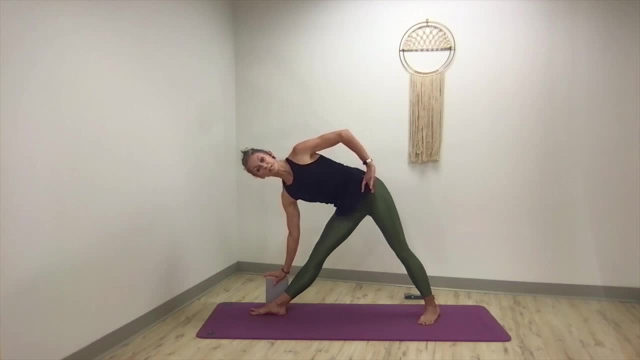 and, as you exhale, rotate, Open your chest towards the front of the room. When you are ready, extend that top arm toward the ceiling. Let it be an extension of your shoulders. Good, Again, head position can be looking up towards your thumb straight. 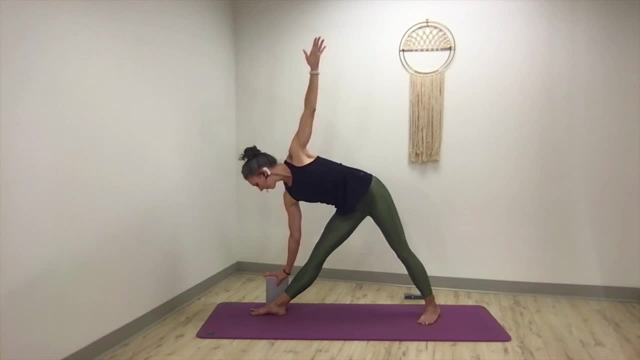 ahead or all the way down to your foot. Take your attention to your feet again. Ground through your heels, Find the intention of engaging in your quads, engaging in your hips and lengthening through the entire length of your spine. Open through your shoulders and let the energy flow. 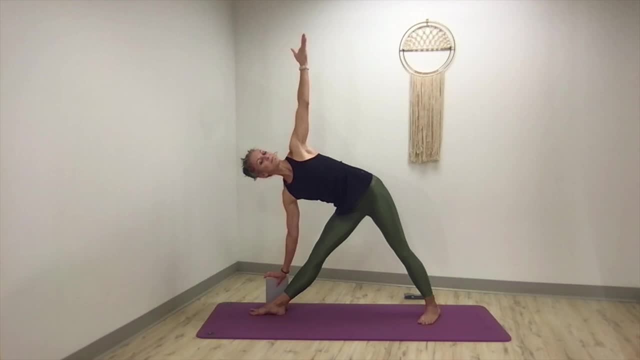 From your fingertips in both directions. Good, One more breath here, Taking your right hand down to your hip and coming all the way back up to stand, pressing through your right leg. Good, You can move that block off to the side. if you have it there, We're going to rotate the feet. 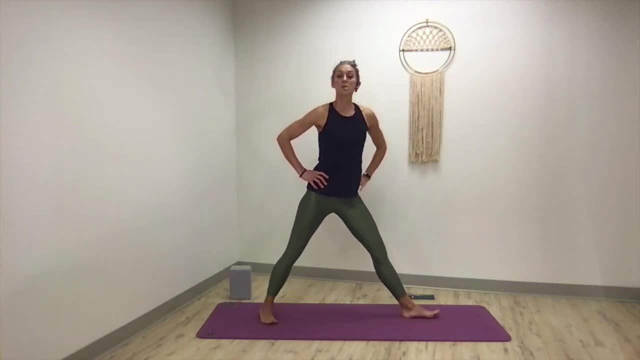 back in. Take the right toes out, left toes in. We're coming to warrior two. Bring your left hip slightly forward. You're going to bend the right knee over the right ankle. And now here, bring your ribs back over your hips And then extend your arms all the way out to the 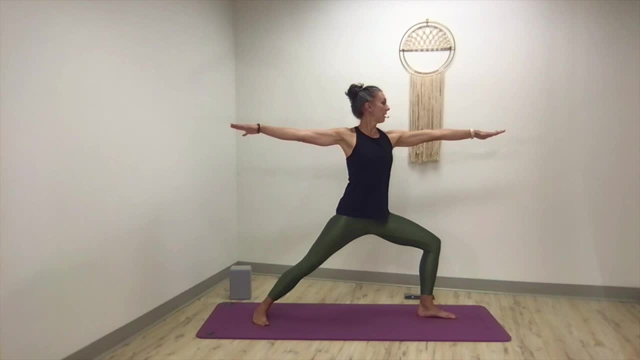 sides. Good Breathe here, Ground down through your feet, down through your heels. Let your left hip come slightly forward and the right hip sink underneath you so you feel the support of your glutes in this position, And then reach out through both fingertips Maybe if you're feeling. 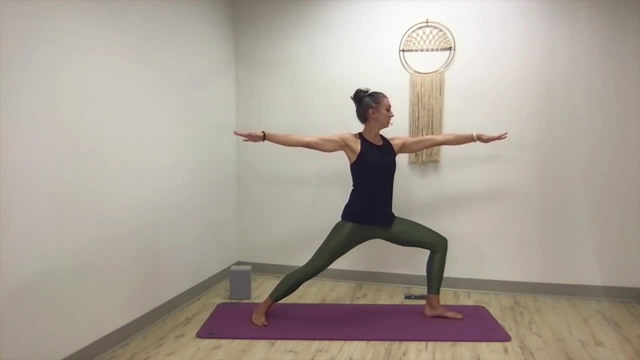 really good. bend that front knee a little bit more, Go a little deeper, Find your breath, Breathe into your back body, Relax your shoulders, Even turn your palms to face the ceiling. Let your shoulders relax And then turn your hands back to the floor with the shoulders released. One more breath here. 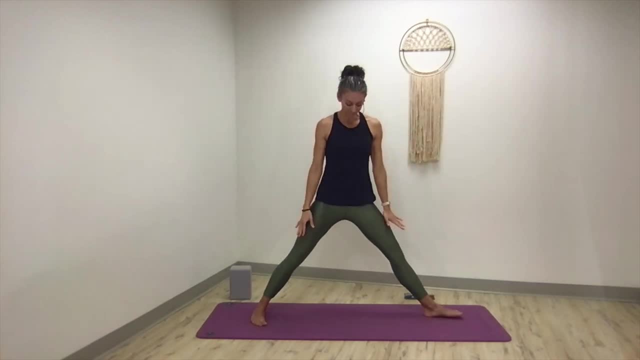 Exhale, Come all the way back up And we'll switch to the other side: Right toes in, left toes out. Bending your left knee over your left heel, Bring that right hip slightly forward- Good- And then drop that right hip underneath you Let. 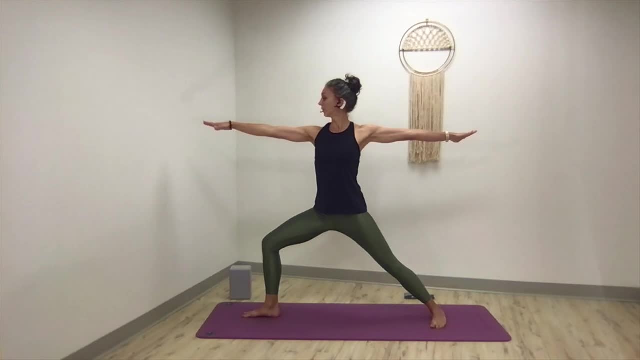 your ribs align over your pelvis And then extend and float your arms out to either side, looking out over your fingertips. Press through the outer edge of your back foot, Deepen the bend of your front knee And check in with your breath. Can you breathe more into your back, Strong, solid? 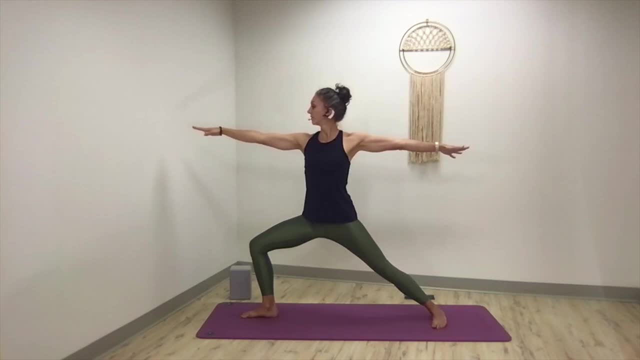 inhales, Strong, solid exhales. And if you start to get comfortable here, can you go a little deeper in that front knee bend, Turn your palms to face the ceiling. Relax your shoulders again. Leave your shoulders where they are. Turn your palms down. Keep that relaxed state in. 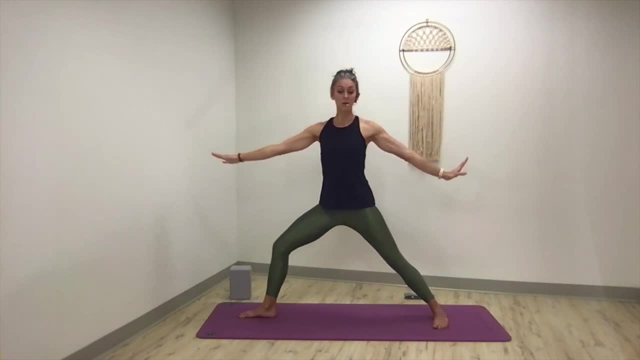 your shoulders, Pressing through your back leg, Exhale, Coming all the way back up. Stand, We're going back over to the other side for side angle. Right toes turn out, Left toes turn in. Feel free to bring a block with you if you need. Put that in front of your right leg. 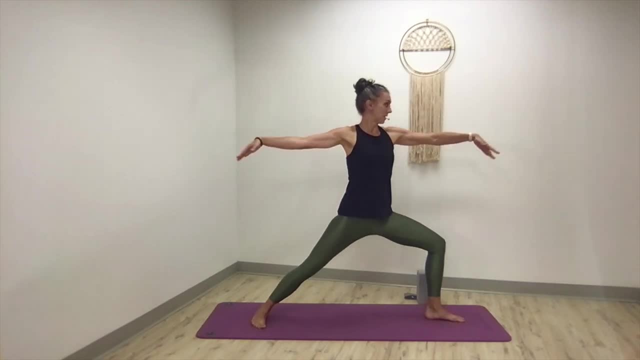 Bending your right knee. we're going back into this warrior two position And here we're going to reach forward just like we did in triangle pose: Deepen that right hip crease And then take your hand and elbow either to your right knee or to a block on the outside of 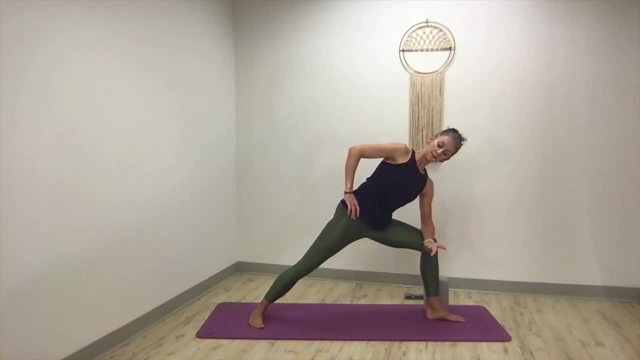 your foot. That's your choice. Press down through your feet, Fire up your glutes, Arrange your hips so you feel some freedom in the core, Freedom in the tailbone, And then take your left arm, sweep it all the way up and over your left ear. Energetically, we want to encourage the left heel to press down and that 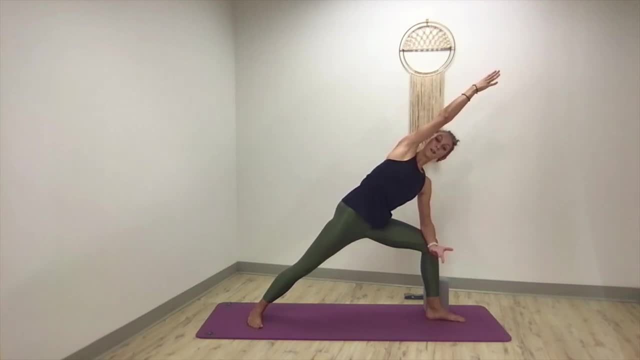 energy to travel up your left leg and all the way through your left fingertips. Deep breaths here Again, bending Right leg A little bit more if you'd like a little more intensity. Two more breaths here. Where can you find the lightness in your pose? 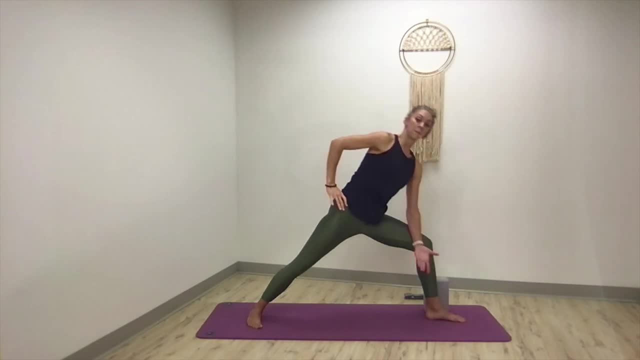 Taking the left hand down to your hip, press through your back leg, coming all the way back up to stand and rotating to the other side. If you use your block on that side, you'll want to take it with you. Left toes turn out, Right toes turn in. Coming into warrior two. 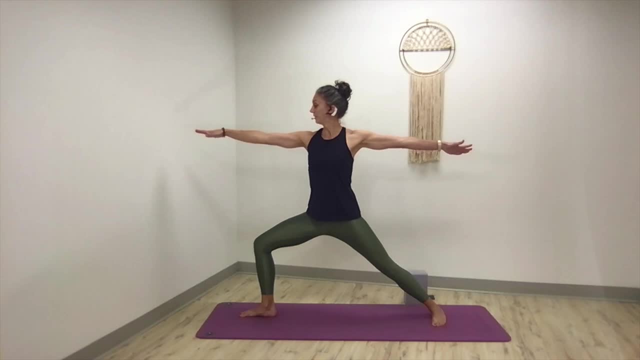 Position to start. Ground through your heels, Ground through your feet, Lift through your rib cage. Now reach forward with your left arm, Take your left elbow down to your knee or to the block or to the floor, Whatever is most accessible to you, And then that right arm circles all the way. 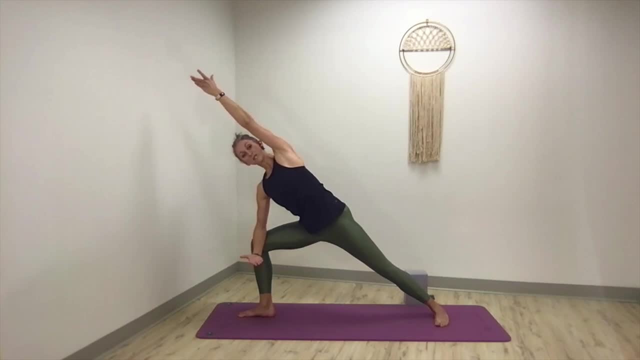 up by your ear So you're making a nice straight line from your right heel to your right toes. Let the weight be heavy in your heels And then drop your tailbone. Let it be heavy so you can feel your glutes starting to work And then lengthening through your spine, Sending that left hip back in space. 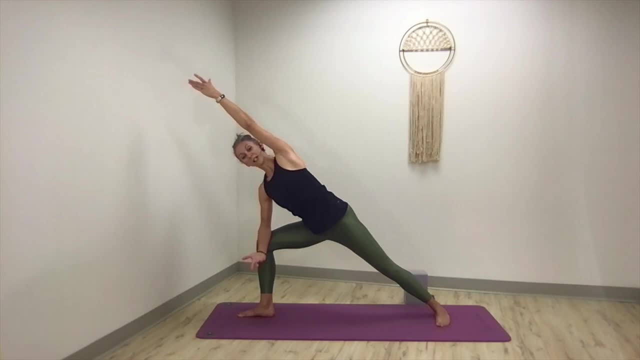 to create a lot of space underneath this left rib. Notice if you've stopped breathing. Go back to your breath. One more breath here, Releasing your right arm all the way down. Press through your back leg, Bring all the way back up to stand Heel toe your feet together. Great. 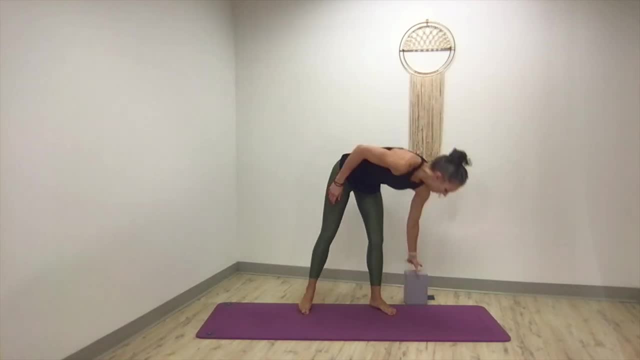 Now we're coming into twisted triangle, So you're going to use your block. We're coming to stand at the top of your mat And we're going to put the block in between your feet. Your right foot will be forward, stepping your left leg back, Spin the heel down, so it's kind. 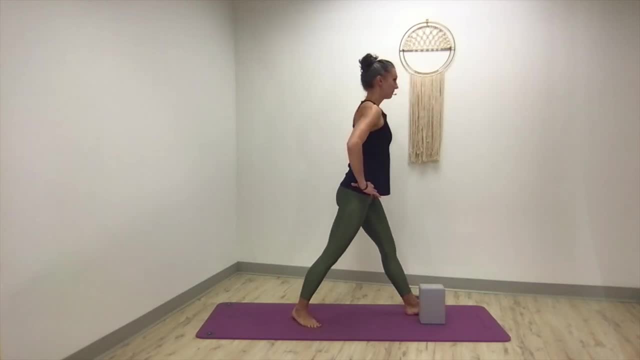 of a shallow stance And we're going to square the hips towards the front of your mat. Take your right thumb into your right hip crease And pull that hip back in space. Reach the left arm up and then reach all the way forward and down to your block. 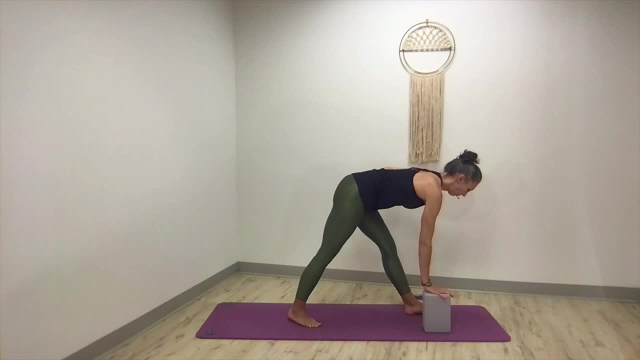 Take your hand to your block, Keep moving that right hip back in space. Keep pressure in your left leg, Deep breaths here, Opening your chest any amount. The key to twisting with osteoporosis is that we have to keep your spine straight while you twist. 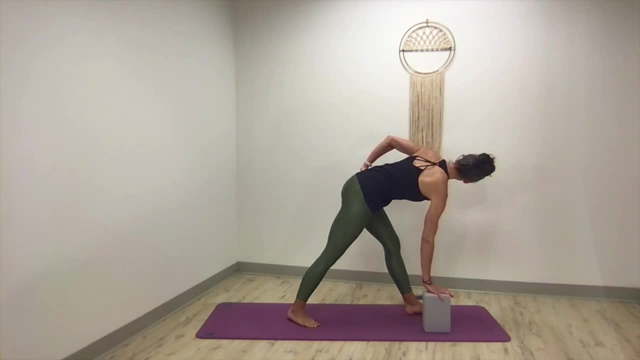 Which means we have to one rotate from our hips but also use our core muscles to help rotate, Not the flexibility of our spine. If you feel comfortable here, reach that top arm towards the ceiling As an extension of your top shoulder. 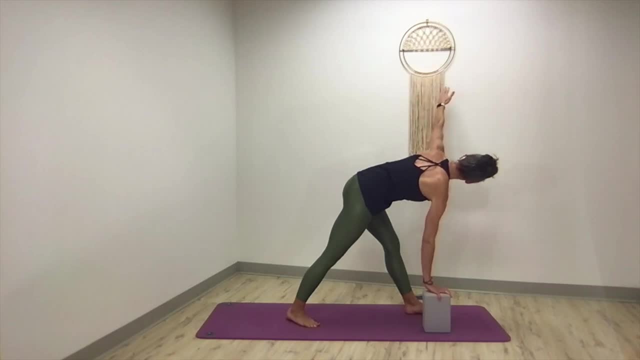 That's if your shoulders are rolled forward like this, Your arm is going to be slightly forward forward. You can also choose to keep the hand on the hip. One more breath here. Press through the back foot and through the crown of the head. Good Inhale, Bring it back to the center. 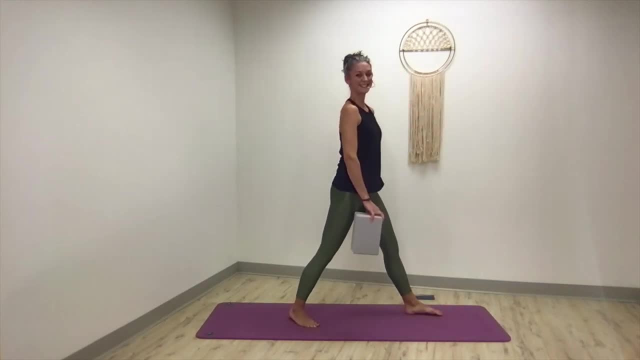 Bring your block with you. Exhale, Come up to stand. Excellent, Switching to the other side So you can just rotate over left foot forward, right leg back. We'll take the block on the inside of your left leg, Squaring off your hips. Your back toes are turned in about 45 degrees. 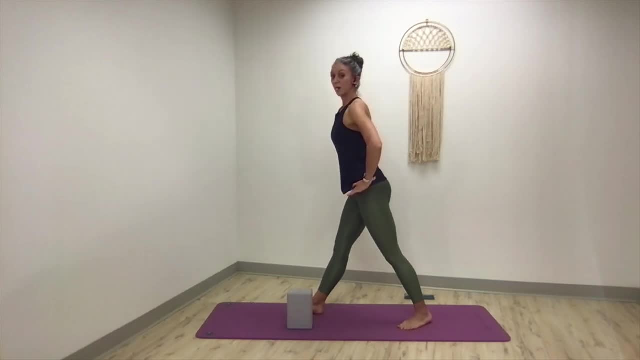 We're going to take the left thumb into the left hip, crease and draw back. So we're squaring our hips off. Right arm reaches up and then reach forward nice and long, keeping that left hip moving back. It's going to want to hike up, so really pull it back. Hand onto the block, Stay. 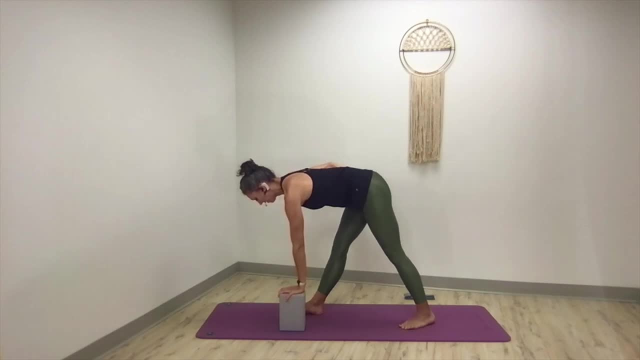 here for a breath. Exhale- Good, If you would like to twist, go ahead and inhale, Lengthen through the spine And then exhale. Twist, Open your chest towards the left, Sending your left hip back, And at the same time, 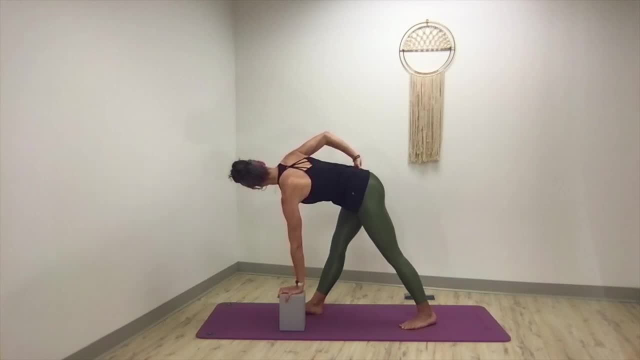 elongating through the spine, through the crown of the head and rotating your chest from your shoulders At any point. you would like to extend that top arm. you may, And bring your head back If you find you're looking down and rounding. see if you can look up slightly. 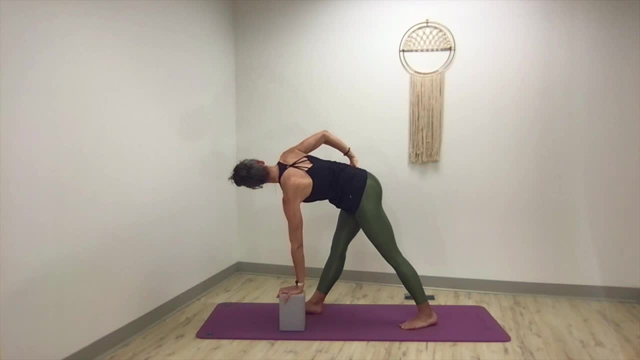 Good, Stay here, Getting heavy in that back heel, Drawing the left hip back in space, elongating through your spine and the crown of your head. One more breath here, Inhale, Returning back towards the center, And then bring the block with you, Press through your. 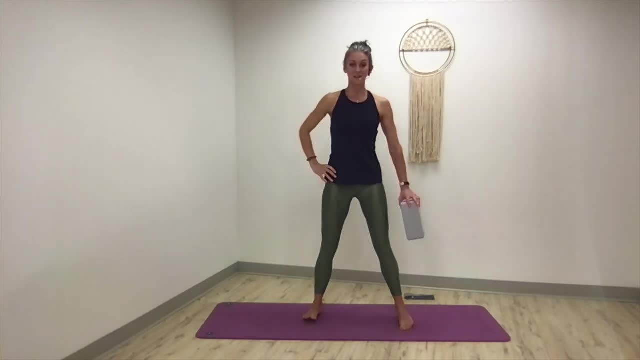 back leg Exhale. Come all the way up to stand Great Heel. toe your feet back together. We're coming down to the floor For locust. Find your position on the floor. Make sure that you have your block and your strap close. 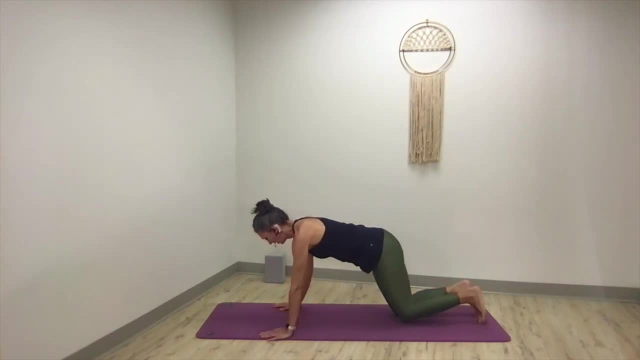 by, We're going to come all the way down to your stomach and your chest. Go ahead and lay your forehead on the floor and bring your arms all the way back by your hips. Relax completely on the floor Now roll the shoulder blades towards each other. Go ahead and lift the hands off the floor. 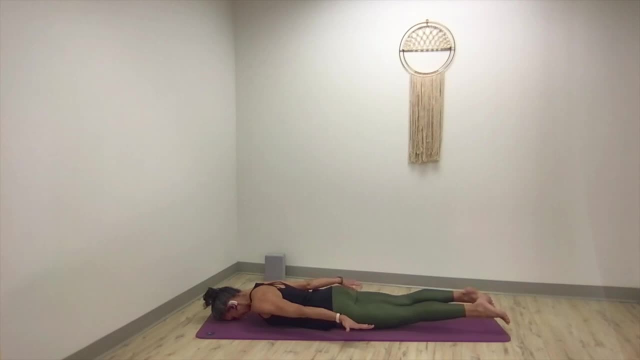 Lift the legs off the floor, but keep the pubic bone pressing down, Keep it heavy, Reach out and up through the legs. Now the final piece is to lift the head off the floor, but let's no jut the chin forward, Let's keep it tucked. 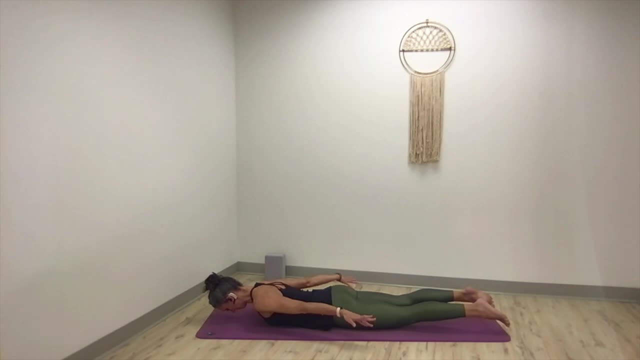 You can bring her gaze down to the floor. Let it be soft And then gently hug the shoulders On your back, reaching through your fingertips In your glute muscle to help you lift your legs. if you feel any pain in your lower back, lower your legs, engage your core, let 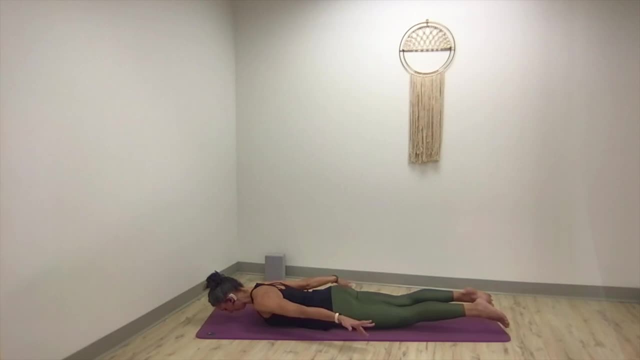 your tailbone be heavy. let's do two more breaths together. feel the expansion of your front body, the lift and the power of your back body. on your next exhale, lower down to the floor, turn your head to one side, resting here. big breath into your back. excellent, we're coming over onto our backs to come to a bridge pose. 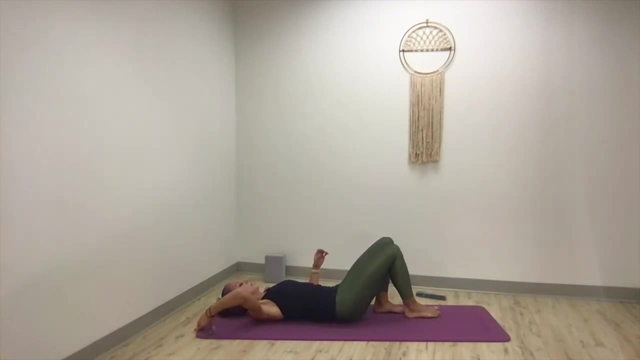 to roll all the way over onto your back. bring your feet underneath your knees, press your hands into the floor, press the little occipital bone, the back of your head, into the floor as well, tucking the tailbone under. let your hips rock back. drive your heels into the floor and 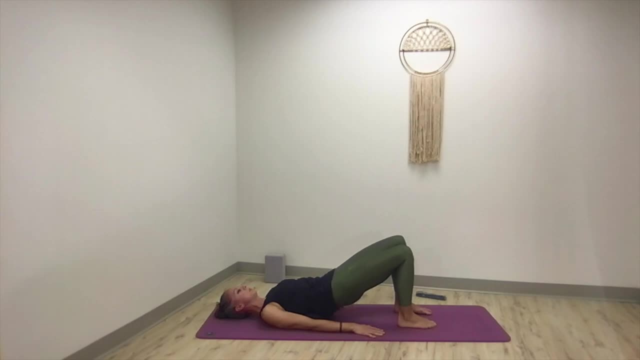 scoop your hips up using your glutes to lift. so we're not shoving from the lower back. we're going to push into the position of the back of your head and lower back. you should not feel this in your lower back. you may not have to go. 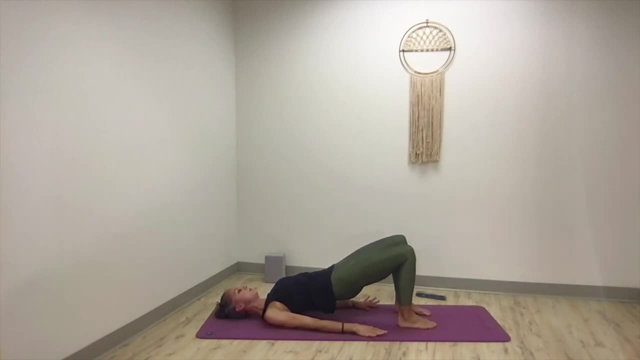 that high, draw the shoulders underneath. you press your arms into the floor and breathe here. press your heels down, engage and lighten up the back of your legs, your hamstrings, your glutes, allow your breath to invigorate. you press the upper back into the floor, hands down into the floor and back of the head. 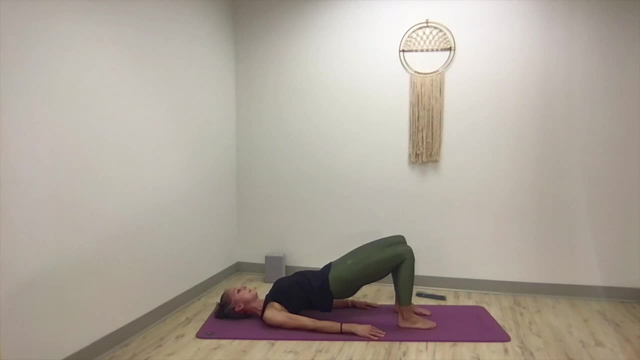 gently into the floor as well to come down slightly. tuck your tailbone, roll down one vertebrae at a time as you come all the way down to the floor to rest on your back. okay, grab your strap and we're going to put this right foot in the belt. 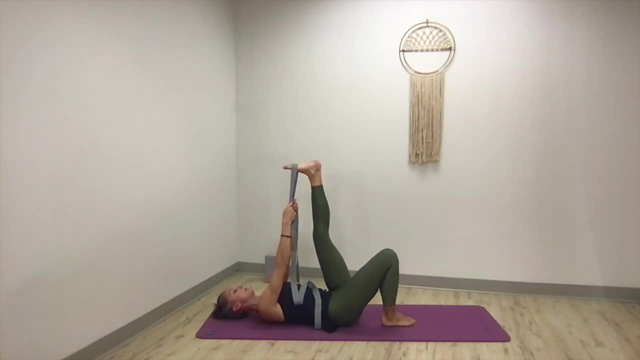 stretch it all the way up towards the ceiling. hold on to the belts. you have the option of putting your right foot in the belt and you're going to put your left foot in the belt and you're going to put your left foot in the belt, and. 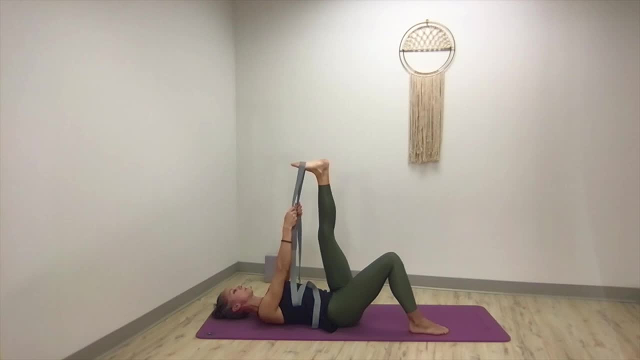 straighten it out whichever is more accessible to you: drop your shoulders down, press through your heel, stay here and breathe into any sensations. drop your right hip away from your right ribs, your right shoulder, relax your jaw, relax your neck and, once it feels good, you can extend your left leg out and 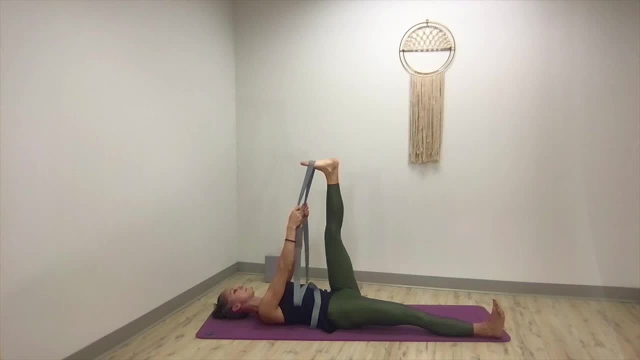 drive through the left heel towards the opposite side of the room and breathe through any sensations. press through the instep of your right foot and then, bringing both ends of the belt into your right hand, take your left hand onto your left thigh for groundedness, bend your knee just a little bit and take that leg. 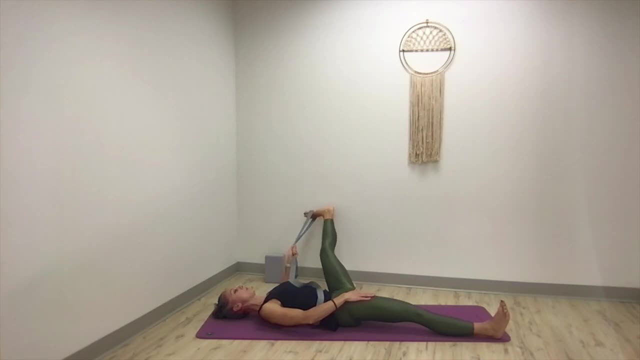 out towards the right so you can bend that right elbow and put it on the floor for a little kickstand. turn your right toes out slightly so you're pressing the heel towards the ceiling. press your foot into the instep and into the band and bring your right leg back into the center. hold onto the belt. good this. 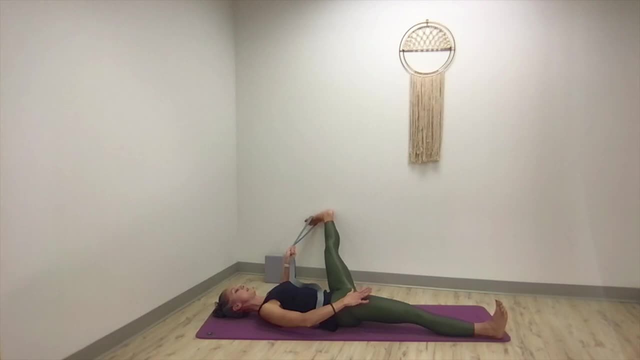 requires a little bit of core engagement as well. and then take your attention to that bottom leg. press through the heel of your left leg and out through the crown of your head, fill your breath expanding into your back body, allow your body to work but also receive at the same time good. bending your right knee, bring it back to the center, hold on to the belt with both hands. 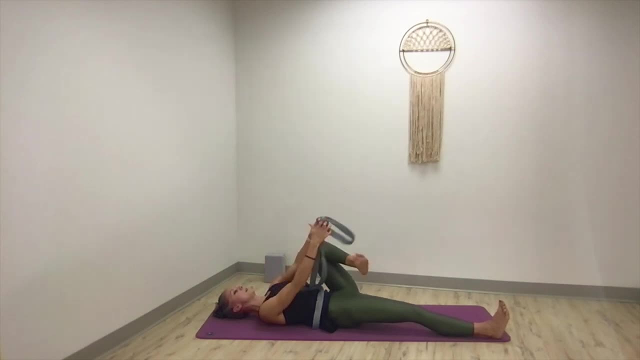 to reset and it'll bend the right knee. bring the belt around the ball of your foot on the left side. we're gonna straighten the leg all the way up over your hip. so option here is to keep this right leg either bent or we can straighten it all the way out if that feels more accessible to you. but you 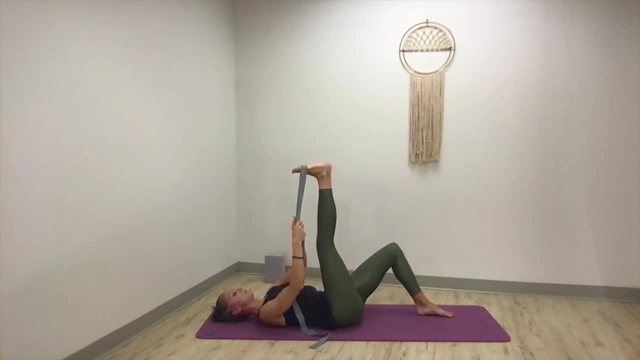 can always leave it bent. all right, flex your left foot now. press through the instep of your left toes, relax your shoulders. hold on to that belt at a level where you're not pulling with your arms, you're just allowing the distance between your foot and your hands to be natural. and if, at some point, 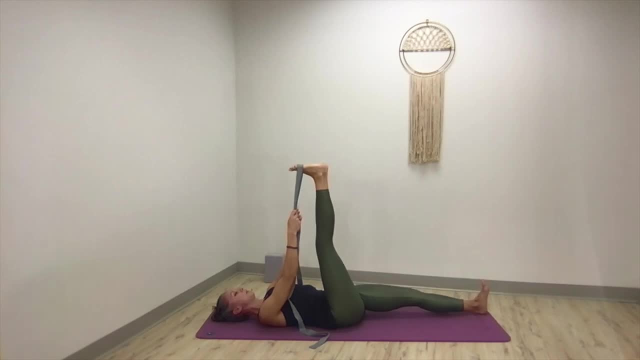 you'd like to extend that bottom leg out. we're going to ground through the right leg. press the right heel away from your hips. find your breath now, your breath to expand into your back body. now. we're going to take both ends of the belt into your left hand. take your right hand on to your right. 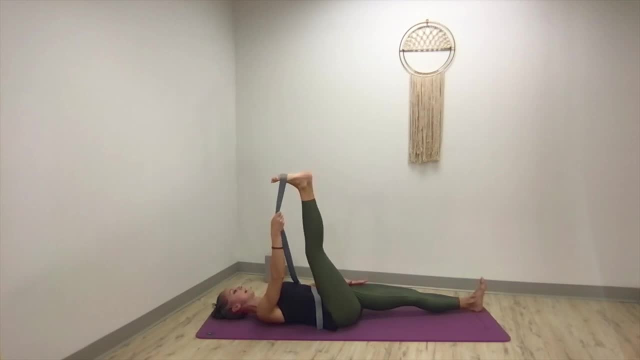 side. ground it down, engage your core and then take the leg out to the left side of your mat so you can bend your elbows. so your elbow works like a kickstand to take it out to the side. turn your left toes down towards the floor and then 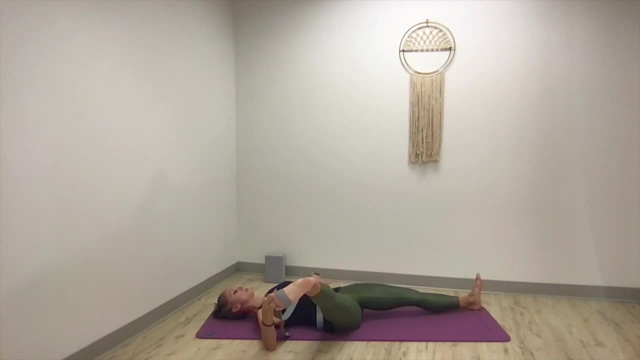 drop your left hip away from your left shoulder, so creating space between the left rib and the left hip. breathe here, drive through the right thigh so you're leaving some engagement in that right leg as I walk. your flips the knee over and sides really broken later in regards to that same pose. 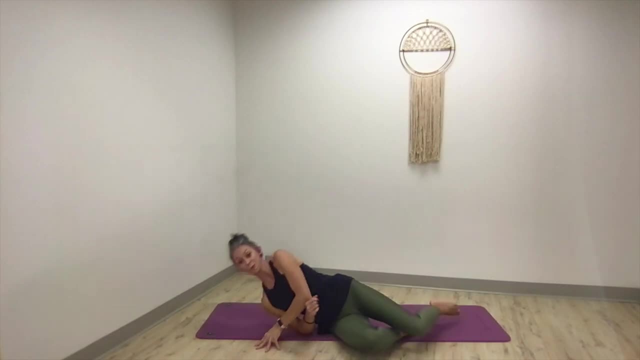 and make sure you prosthetic toes are bent to connect and then fold out the right knee into your forefoot leg. extended out, your right knee will come into your chest and bring that right knee as close to your hips as you can so it's very, very close extend. 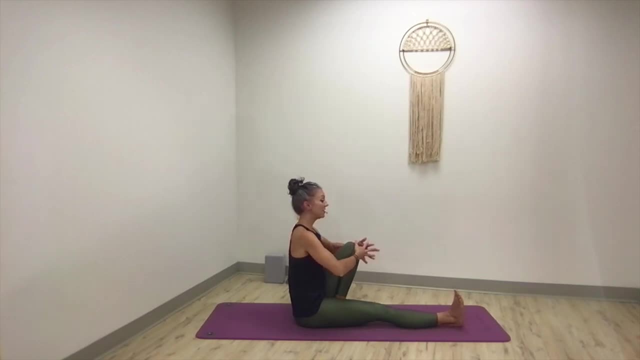 through your left leg and then lift your chest forward. so this might be where you stop. if you have a lot of tightness in your lower back, you can just work here if you would like to twist. we're going to hold on to the right knee with your. 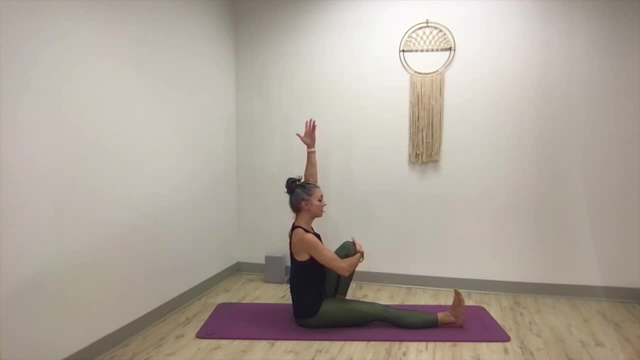 left hand, reach your right arm up, but this isn't an important step, especially for osteoporosis. we want to stay straight and lifted in order to stay safe in your osteoporosis twists. alright, so we're gonna inhale, reach up and then exhale. rotate through your upper back and through your chest. make sure your 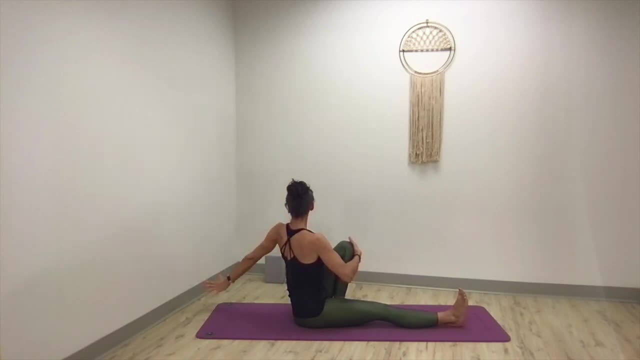 lower back is staying nice and straight and then reach your arm all the way back behind. you tent your fingers on the floor and open your chest toward the right breathe into your mid back. you are staying as compact as possible through your lower belly to your right thigh and letting the twist happen from your upper back, and this is a safe twist. 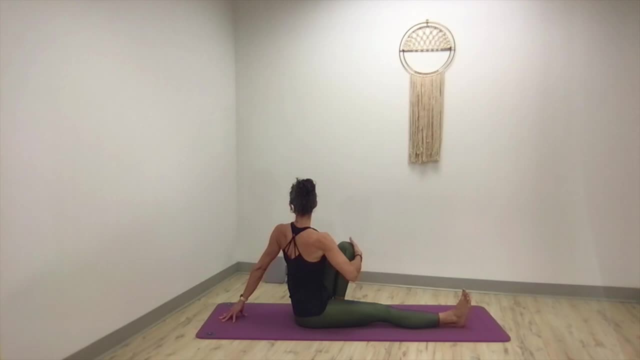 for osteoporosis if we are staying upright. trouble is when we get into twists and we're rounded like this. so stay upright. you can opt to turn your head all the way towards the right, even turn your eyes towards the right side of your mat. much as they can inhale, grow taller through your spine, exhale, rotate and 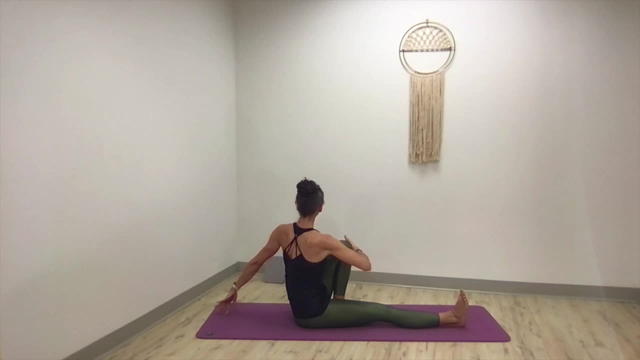 twist, inhale, come back through the center, reset, hold on to your knee and then extend your right leg all the way out, bringing your left knee into your chest and again hugging that heel back towards your hip as much as possible. now grow really tall through your spine, bring your left knee towards your chest. 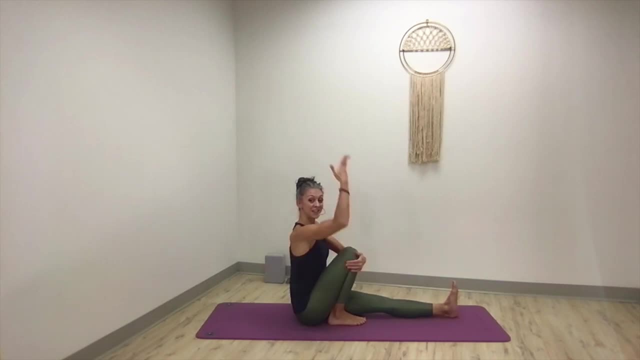 hold on to your left knee with your right hand. left arm reaches up overhead. get really tall and rotate through your upper back. let your left hand float down to the floor. tent your fingers on the floor as you inhale. lift your chest as you exhale. rotate towards the left. continue to draw the left knee into your 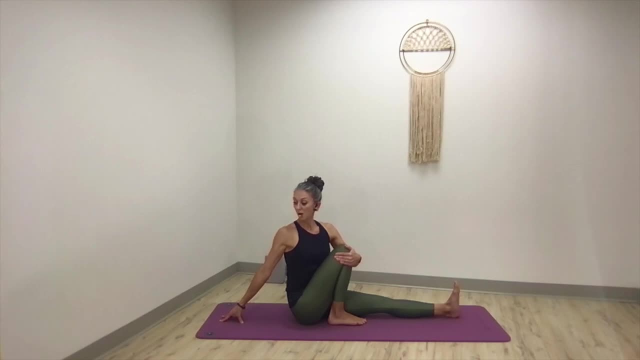 chest as you're rotating, staying long through your spine. you and we don't have to pull ourselves into this rotation. we want to get there gradually and naturally. so go with your own range of motion from here: as you're inhaling, grow longer and as you're exhaling, rotating more, maybe taking your. 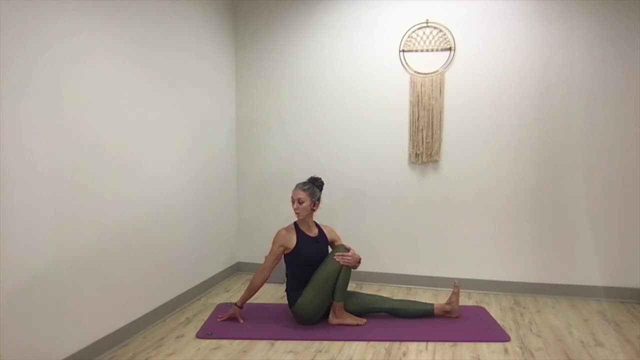 gaze all the way to the left side of your mat. one more breath here. inhale and exhale, rotate, inhale gently, come back to the center, reset, hug the left knee into the chest and then come back to the center, and then come back to the center. 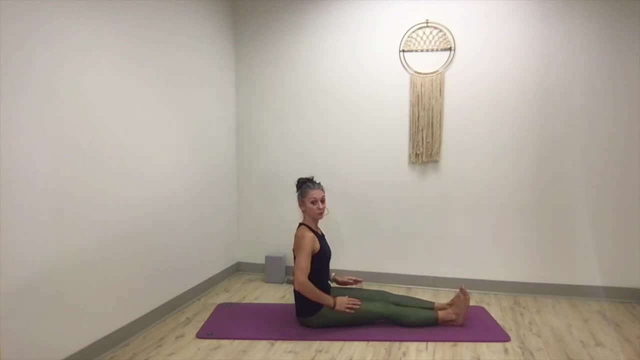 and then extend your legs all the way out on the floor. just go ahead and bounce your legs a little bit, wiggle out your feet a little bit. now we're coming into a bent knee twist. we're going to start with the right leg crossing over, so 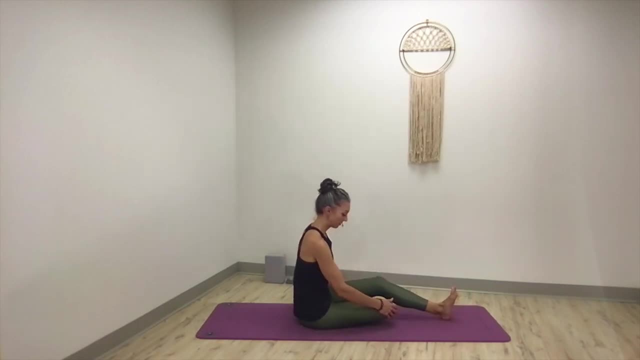 we'll take the left leg and cross it underneath you, take the right knee and cross that one over the left, so your left heel is right by your hip on this other side, and then bring your chest towards your knee, get nice and tight and nice and tall, press through your hips, lift through your spine, find this. 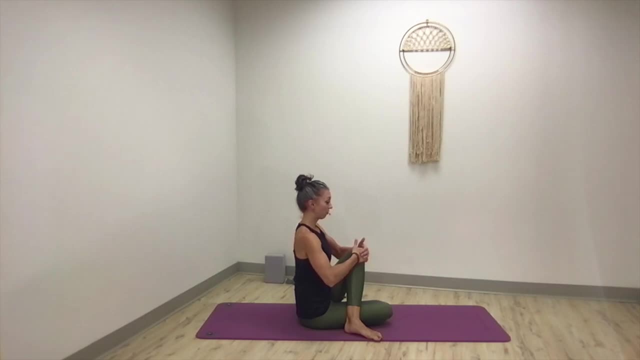 position first, before we start to twist: ground through your hips, ground through your feet with your left hand, grab onto your right knee, lift your chest, reach your right arm up towards the ceiling, grow taller through your spine and then exhale. rotate out to the side and bring those right fingertips all the way to. 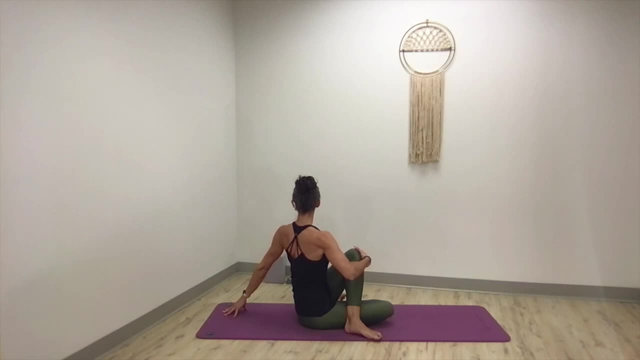 the floor. let there be heaviness in your sit bones. rotate your chest towards the right side from the upper back, breathing in. bring longer exhaling rotating more to the right. bring your attention to your feet. press your right foot into the floor to potentially help you get a little more rotation. one more breath. here we're. 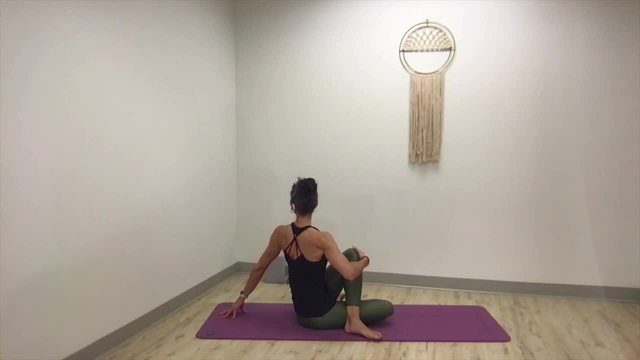 longer through your inhale. exhale open to the right unraveling. coming back to the center, straighten the spine with the right knee to the chest and then extend both legs all the way out to reset and shake your legs and then we'll take the right leg underneath the left. bring it up by 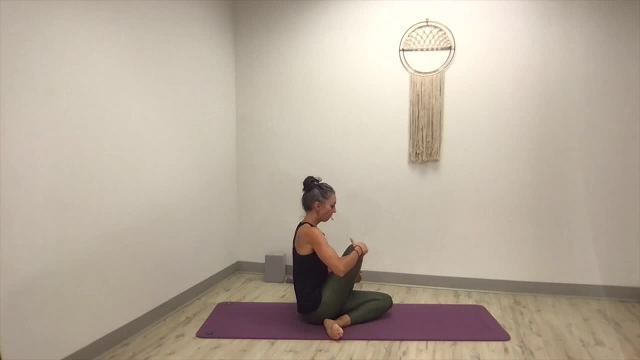 your left hip and then the left leg comes over the top of the right leg. sitting tall, draw your left knee into your chest. press your sit bones down into the floor, taking the right hand around your left knee. reach the left arm toward the ceiling as you exhale. rotate open through your shoulders. draw that. 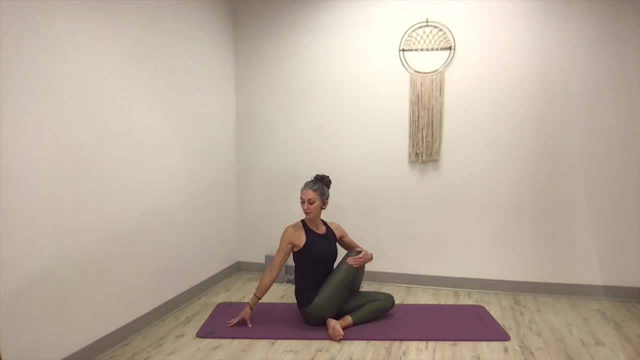 left knee into your chest. fingertips float down to the floor as you inhale. lengthen through your spine as you exhale. rotate open towards the left. make sure your spine is staying nice and straight, especially in the lumbar spine in your lower back. if you're not able to stay straight, you can come back to a 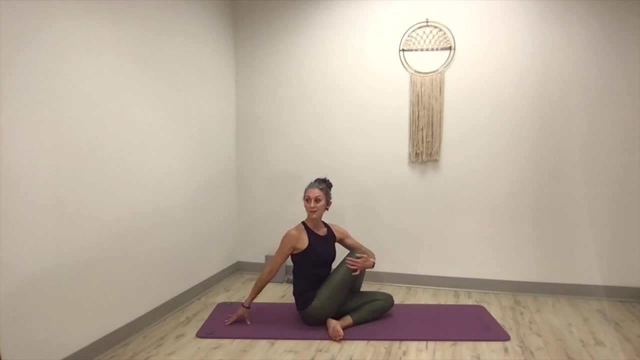 gentle, twist here. press your left foot down into the floor in the front to help you initiate that twist and rotation even more as you inhale. lengthen through your spine as you exhale, rotate deeper, using your deep core muscles to help you rotate and twist through your upper back. inhale unravel. come back to the center, sit tall. 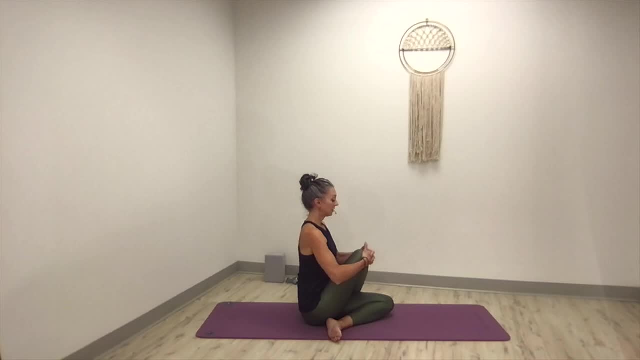 draw your left knee into your chest and then lean back into your hands, extend your legs all the way out, bounce your legs and we're coming down to chevalier basana. roll down to your side and lay all the way onto your back. no options for shavasana, who would like to put a blanket underneath your knees. you can, or. 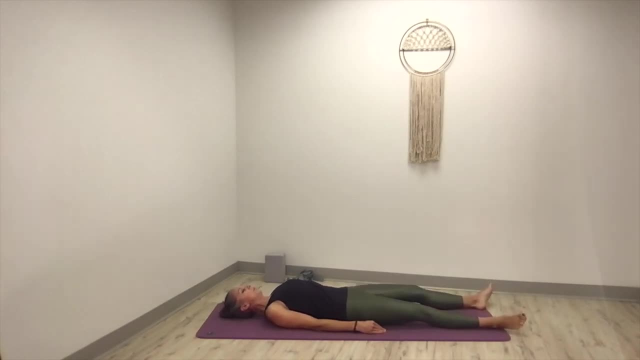 you can just extend your legs all the way out. let your feet roll open, let your arms roll open, the back of your palms laying on the floor, draw your shoulders down your back and down your yoga mat. let the back of your, your head, fall into the floor. so the small occipital bone at the back of your 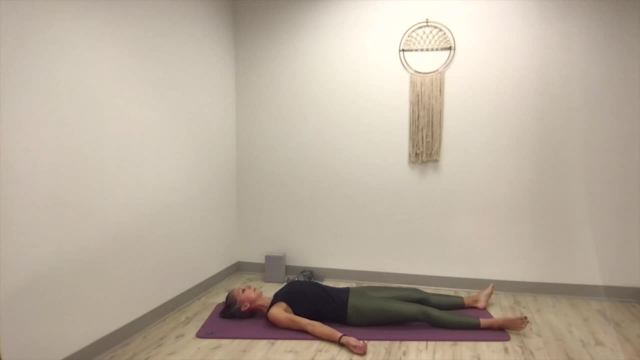 head is heavy on the floor and if you would like close your eyes, allow yourself to settle here. this is your body's chance to really integrate all of the work that you've done thus far. if your mind starts to wander, just bring it back to the breath. 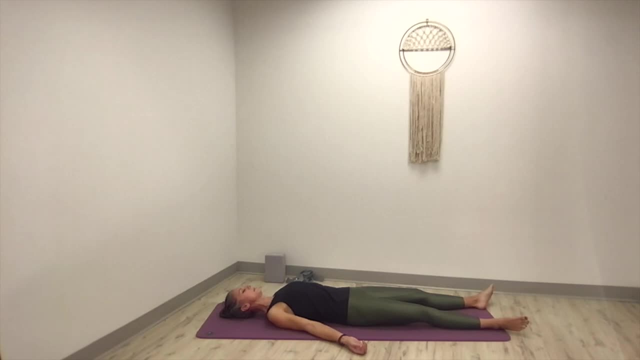 resting in shavasana and all the parts of your body that are touching the floor to fully relax and release. I'm going to be silent a short bit, but I will let you know when it's time to come out of the chest. Slowly, begin to deepen your breath: Longer inhales, longer exhales, maybe even parting. 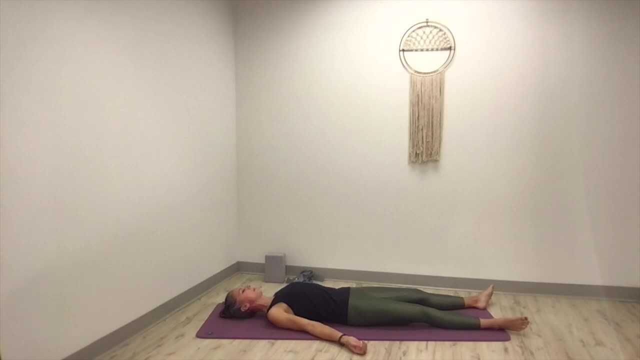 your lips to breathe out, Wiggle your fingers and your toes. Your eyes are closed. I invite you to keep them closed- And then gently bring your hands together, Bring your feet flat to the floor, Rolling to your right side, Resting in a fetal position. 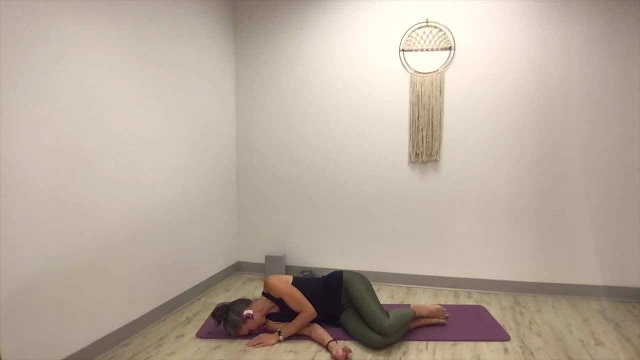 Let the forehead come down to the floor. Just rest, Pressing your hands down into the floor. let your head be heavy and come up to a comfortable seat with your legs crossed. Take your hands onto your knees. Your eyes are still closed. You can leave them closed.